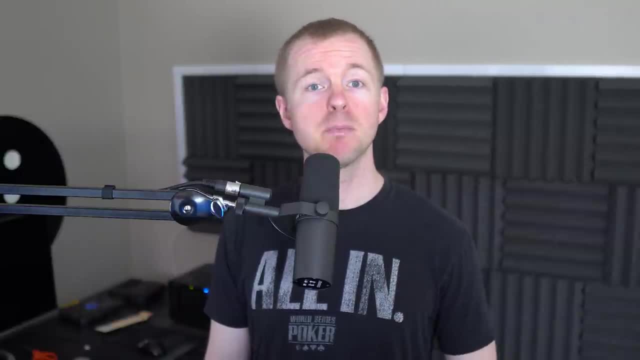 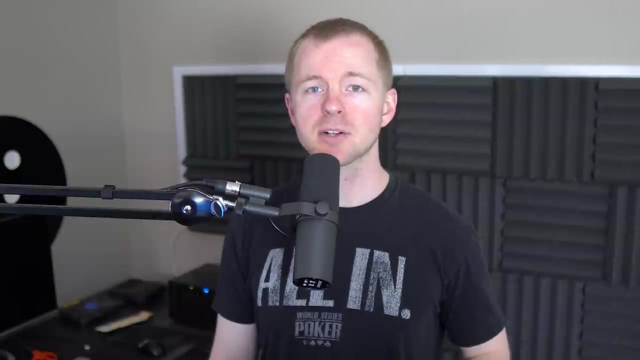 that will always be consistent in security is that new bugs and vulnerabilities are found every day. Being able to identify vulnerabilities or weaknesses in our networks and track them throughout their life cycle until they're resolved is crucial to keeping a network secure. After all, attackers have the same bulletins and vulnerability release information that we do. 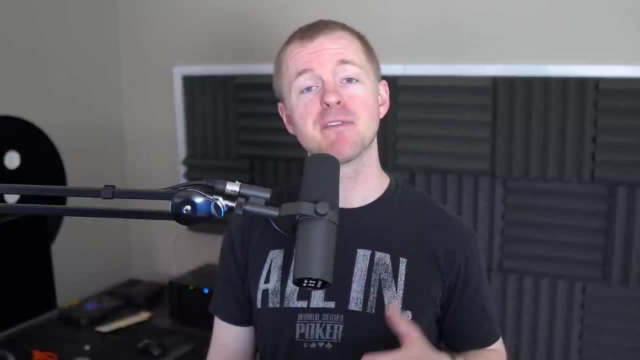 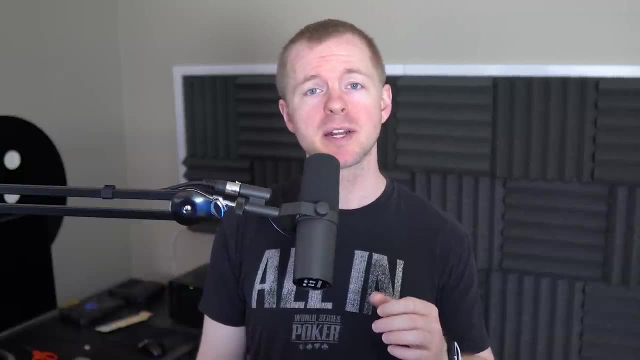 so it becomes a race to fix that vulnerability before an attacker can exploit it. Have you ever heard of the CIS controls? The CIS controls are the same as the CIS controls, but they're are critical controls that an organization needs to secure their network: Continuous vulnerability. 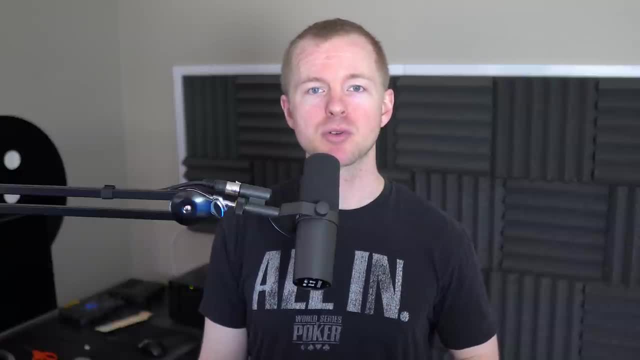 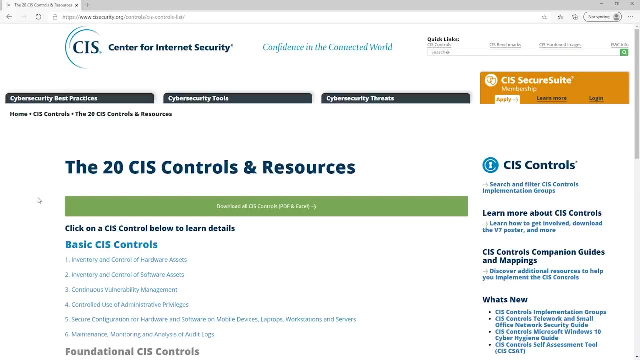 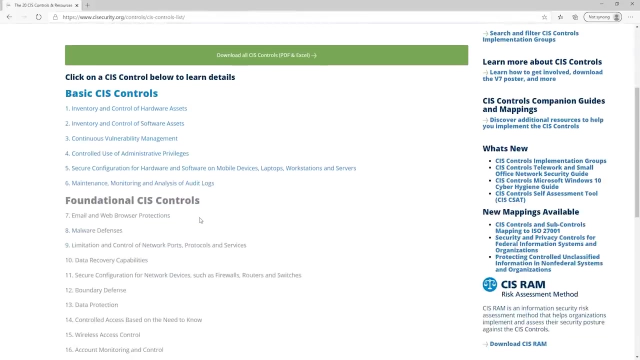 management happens to be the number three critical control that an organization has to have on their network. If you haven't heard of the top 20 controls, what you can do is go to CISecurityorg and they have a list of all the different controls if you want to look more into this. 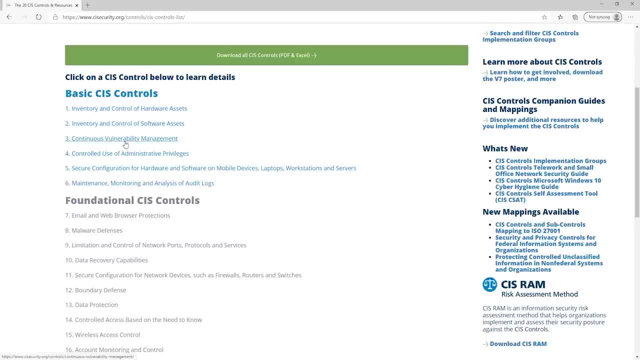 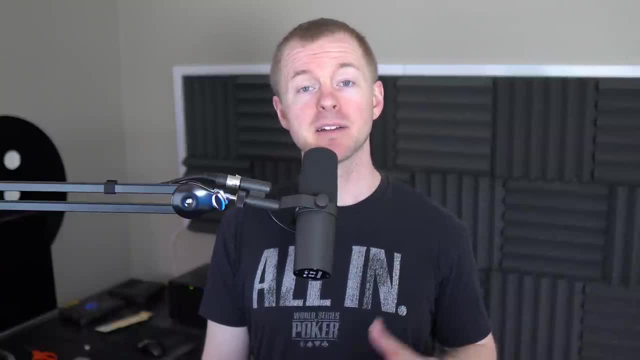 But right here at number three, we have continuous vulnerability management. Let's be honest, as you'll begin to see, the vulnerability management life cycle can take a lot of time and resources. in order to be successful, We have to know the systems that we have on our networks. 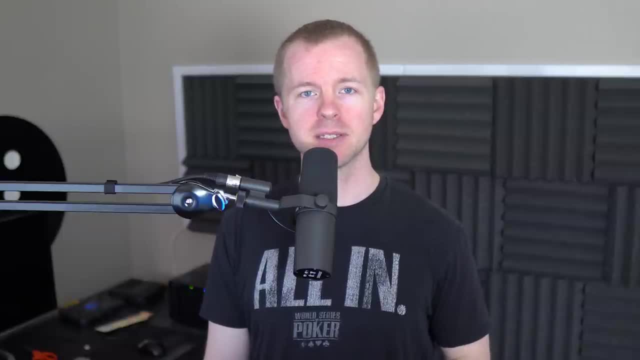 then we have to go scan those systems and identify vulnerabilities. We have to determine the vulnerability severity, so how likely it is to be exploited, and then we actually have to track that vulnerability through its remediation. Luckily there's commercial tools that exist. 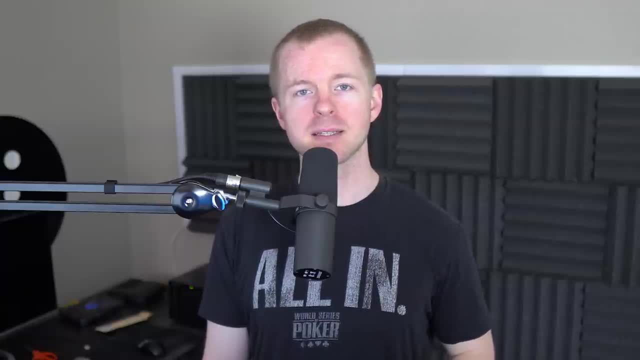 to assist us in the vulnerability management process. In this particular video, we're going to cover Nessus, which is a popular vulnerability scanning tool. Nessus has two different components that make it actually work. First, we have the client, and this refers to that web interface that we actually use as the administrators or users. 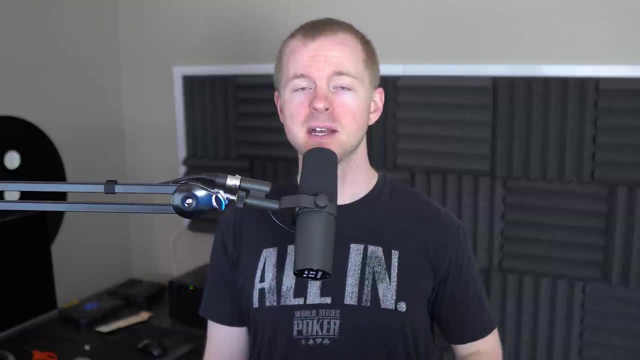 and we can interact with the system to schedule scans, generate reports and all kinds of other features. The other component is the server component. This is what actually performs those tasks and then it sends the results over to the web interface or the client With vulnerability. 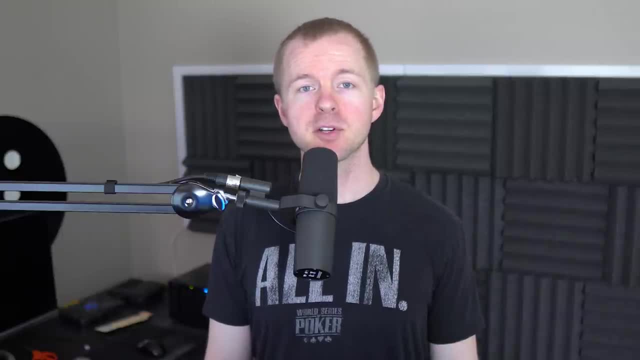 scanning. there's four major steps. The first step is port scanning. This is where the scanner is going to actually go out there, determine which hosts are alive and which ports are open on those hosts. Then we have service detection. This is where Nessus is going to send out probes. 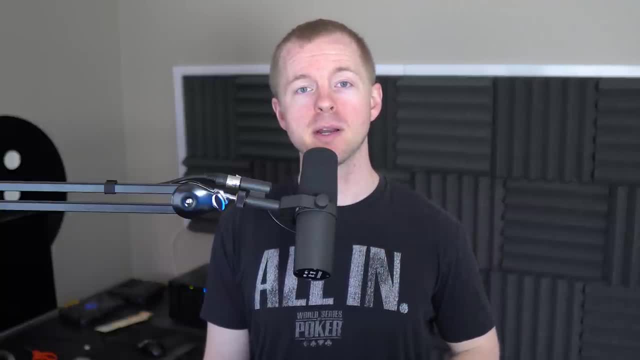 to find out which application is running on that port, the version number and the actual name of it. Then we have vulnerability identification. This is where Nessus is going to send out probes. Nessus is going to compare what it discovers about each service detected on each host. 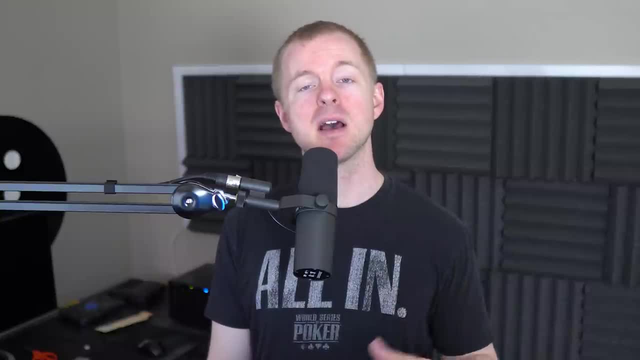 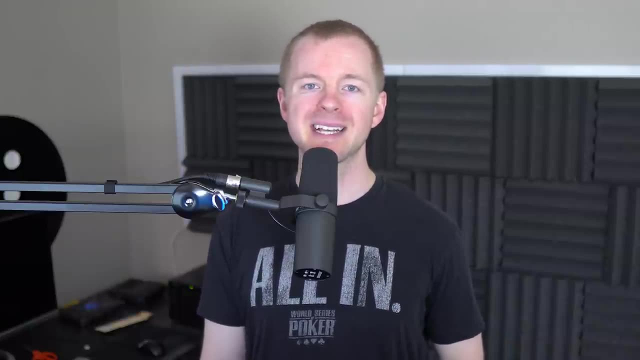 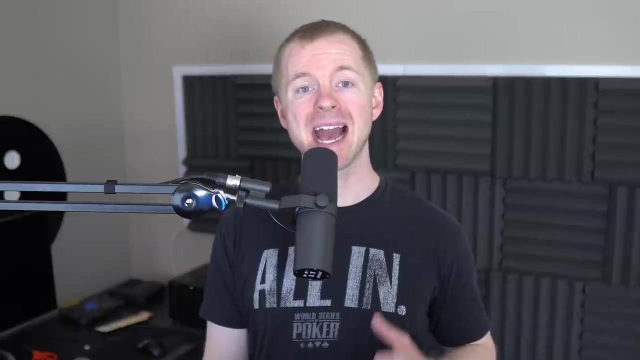 and then it's going to actually compare it against its database of known vulnerabilities of those applications and version numbers, And then, finally, we have the probing step. This is where Nessus is actually going to try to further identify if there's false positives or identify if that vulnerability actually exists. Now that we know some of the basics, 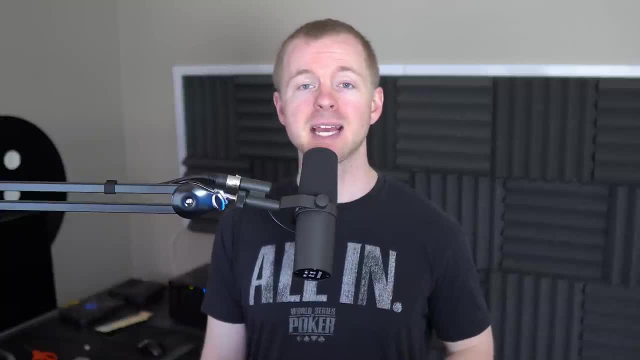 about vulnerability management and vulnerability scanning. I want to actually take you through the product by installing it and running some scans so you can actually see what it looks like. For this demo, we're going to be using the free non-commercial use license that you can also use. 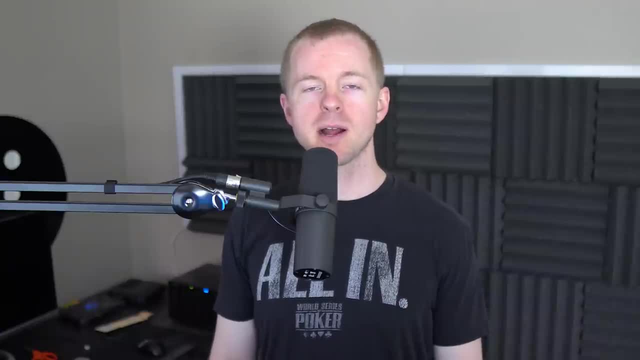 at home if you want to practice along Before we get started. I want to make sure that we're on the same page as far as a disclaimer. So everybody say it with me: I will not scan networks that I do not have written permission to scan. Okay, we agree, If you scan networks. 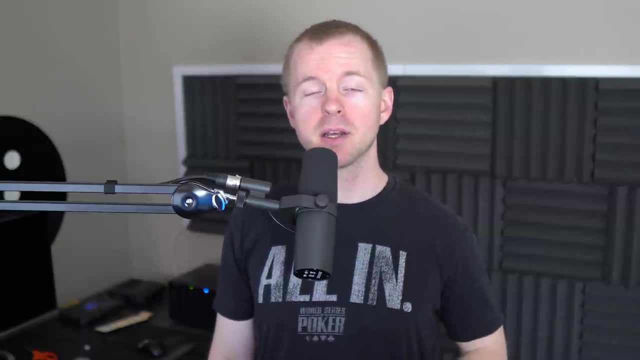 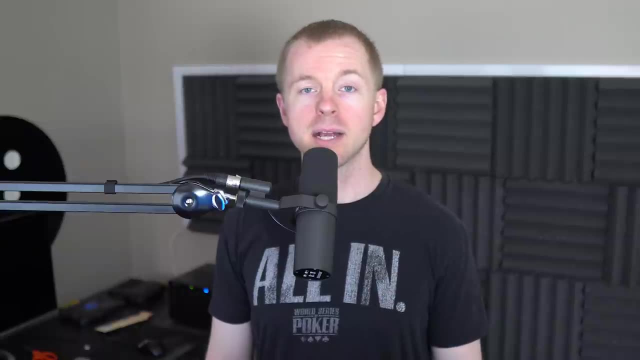 that you do not have permission to scan, you can actually get into a lot of legal trouble. So make sure that you're only scanning systems that you have permission to scan. All right, so let's go over to the computer now so we can install Nessus. 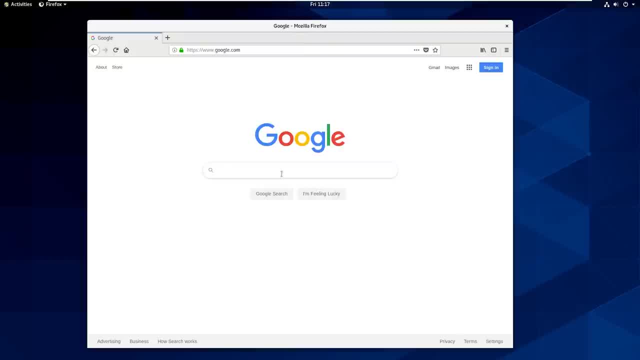 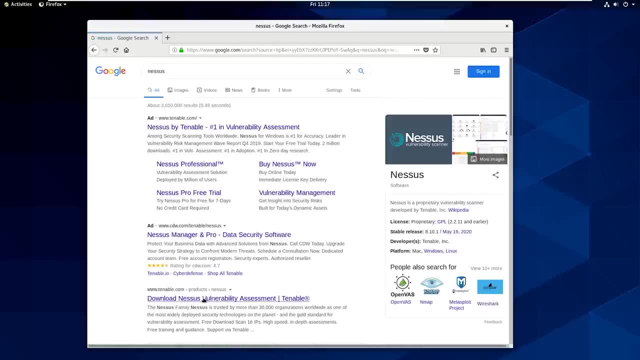 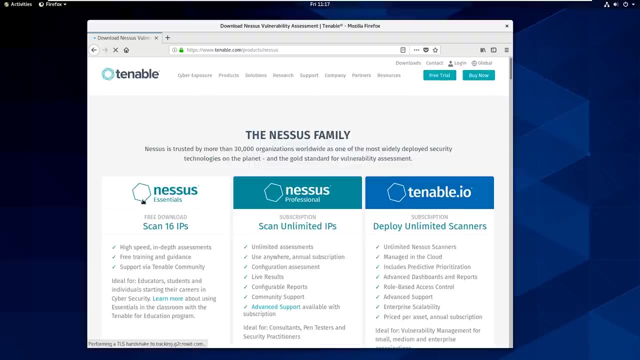 So the first thing that you're going to want to do is go to Google and search for Nessus, And Nessus is made by Tenable, which is the producing company here. We'll click this first link And the Nessus Essentials is the one that we're actually going to use for our home use. 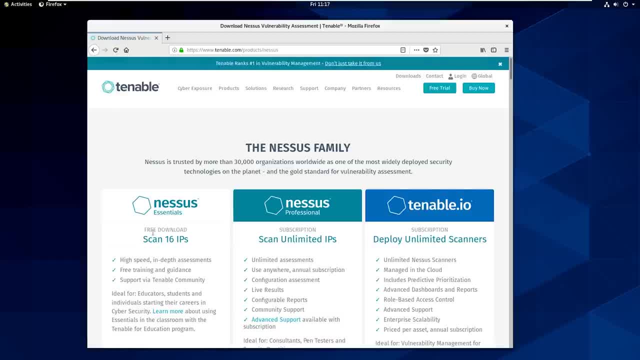 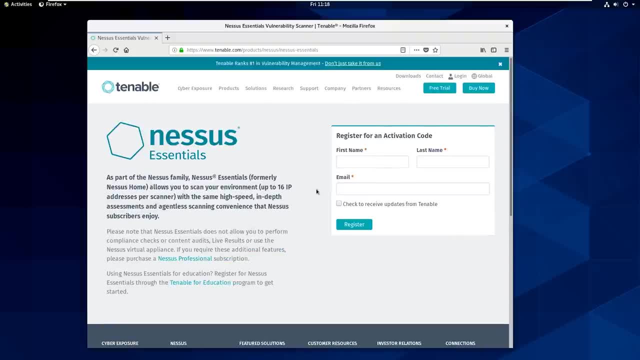 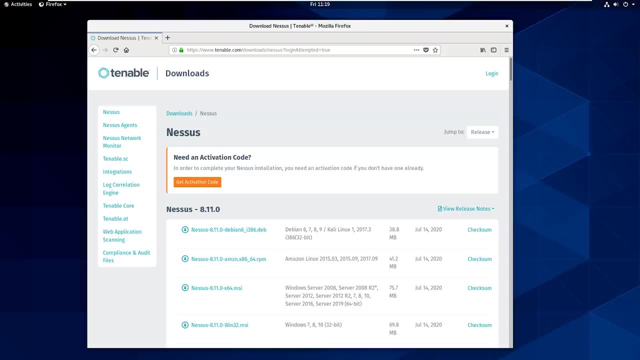 You can see that there's a few other options that you would use in an actual corporate environment. We'll scroll down here and we'll go to download. So you will have to actually register to get an activation code from them. So I will go ahead and do this and then I'll check back in Once we enter. 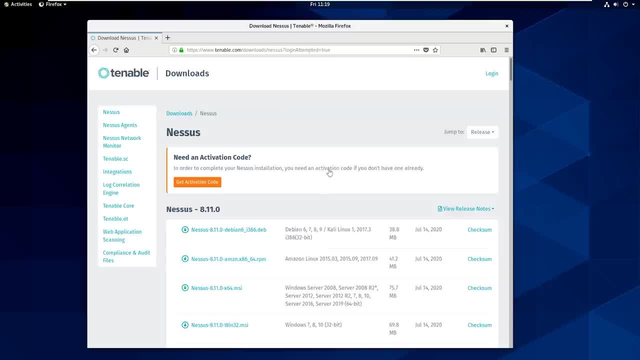 our information, it will take us to the download page And then we just have to pick the version that we want to use. So we're going to go to the download page And then we just have to pick the version that we want to use. 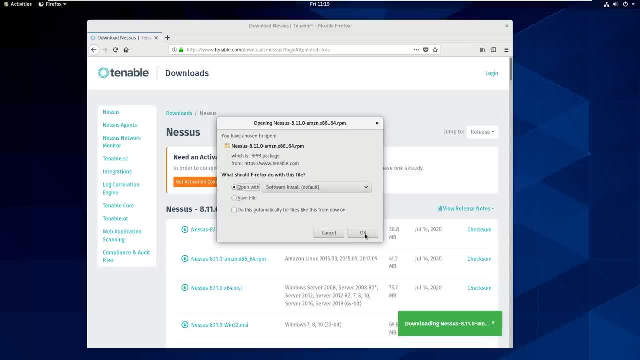 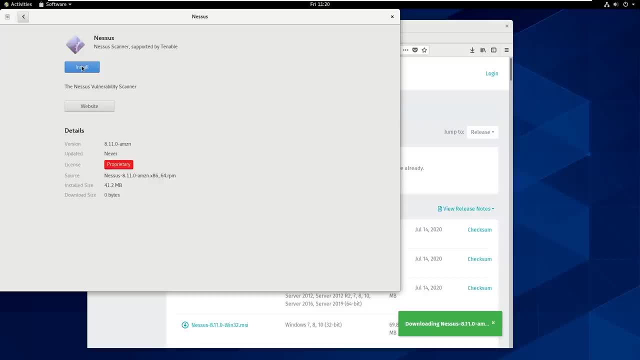 Set the terms And go ahead and install. I am running CentOS here, so yours might look different depending on which operating system you're running, But again, we're going to install it. I'll enter my password here And now that we have it installed, we need to go ahead and start it up here. 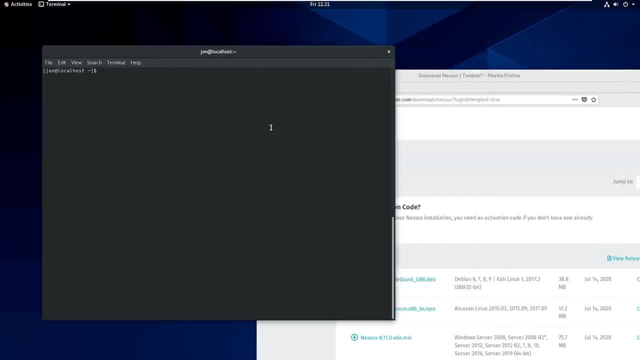 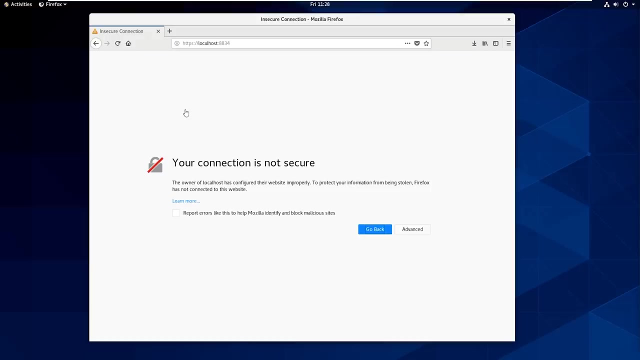 So I already have a command line here. I'm going to go ahead and install it. Command prompt window open back here, And so I will change to root And start the service. All right, great. So Nessus is started now. So when you're actually going to connect to Nessus, 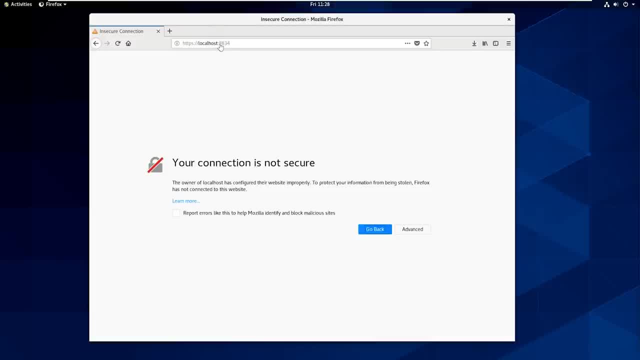 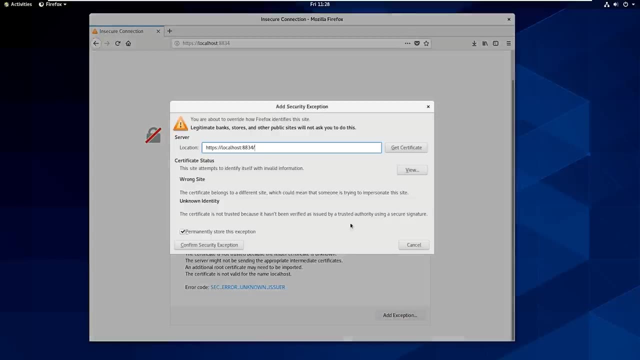 after you've installed it you need to go to your local host And then port 8834 is the website. You'll get this error because it doesn't have an official signed certificate. So hit advanced And then add exception And confirm security exception. 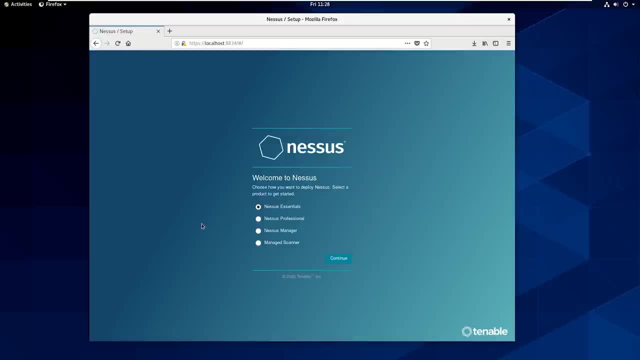 Now we'll be brought to this web page where we need to select our specific version. Again, we did Nessus Essentials, So continue. And then we already have an activation code. So we can skip this step And we'll enter our activation in here. So I'm going to enter mine. 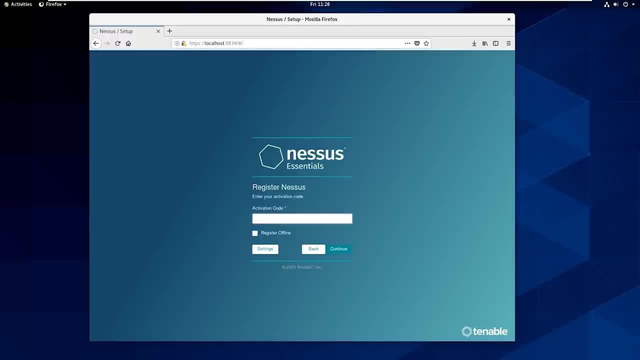 in and then hit continue, And then I'll check back in once. we're done with that. So we're done with that. So we're done with that, So we're done with that. Now that we've entered our activation code, we need to create a user account. 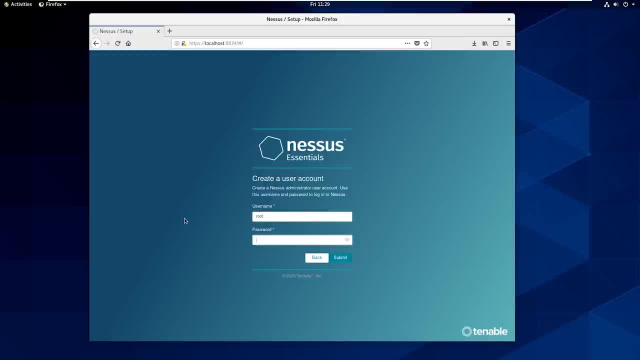 So I'm going to create the username root And the password will be super secret, And then hit submit. Now, this account is the account that you'll log into when you need to run a scan. What it's going to do now is it's going to go ahead and download the plugins. 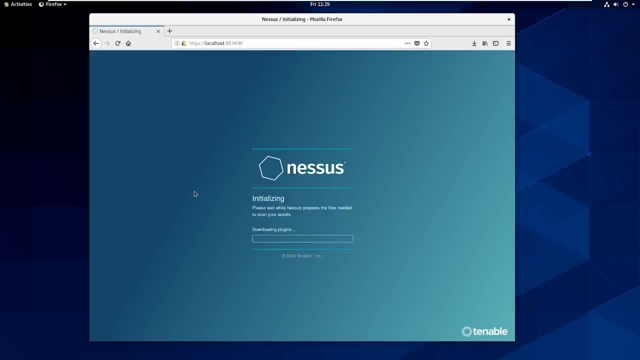 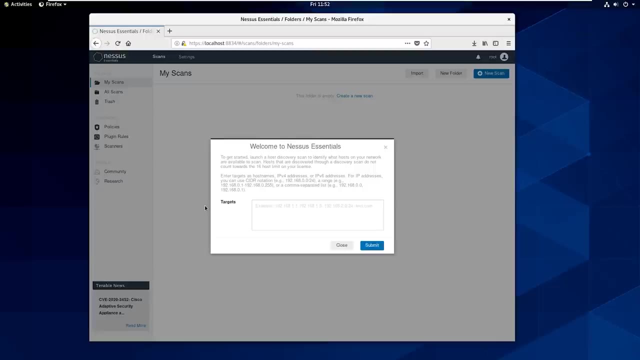 It's going to update itself so that we have all the available signatures and the most up-to-date database for when we perform our scan. So we will let this run And then we'll check back in once we're done with that. All right, And now we have successfully installed Nessus to our local system with the Nessus. 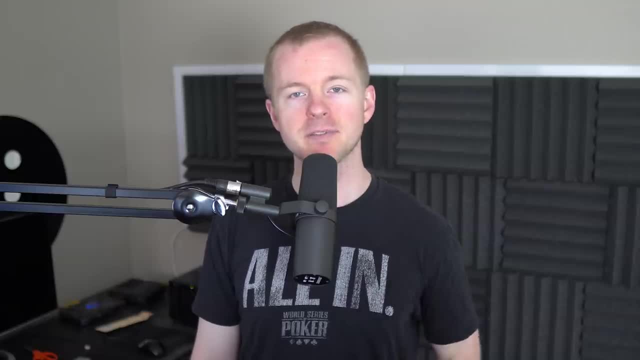 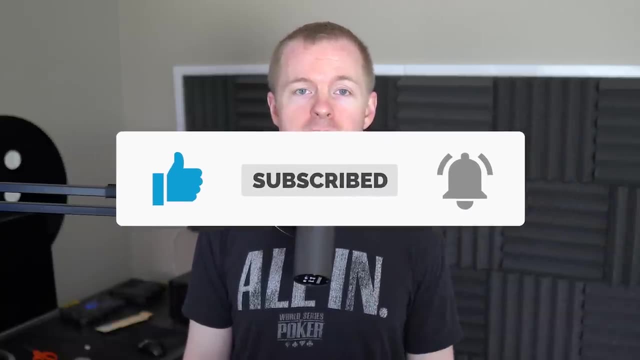 Essentials license. I hope that you're enjoying the content in this video so far. If you are, make sure to hit the thumbs up to like this video And if you think of any questions, let me know down in the comments section below. Also, remember that this training and full courses can be found on my website at: 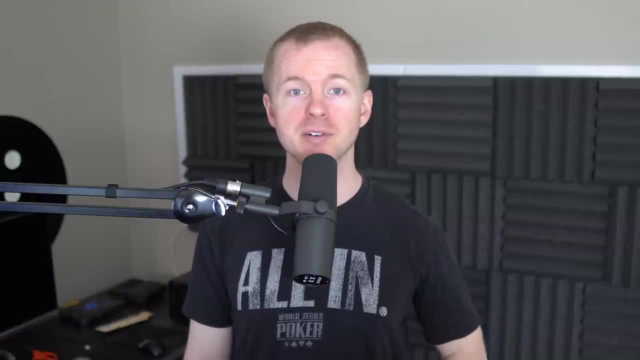 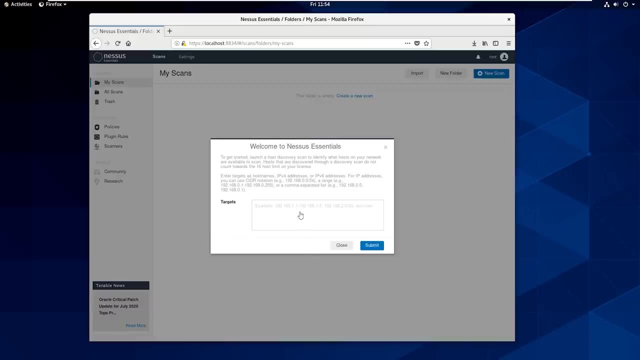 johngoodscom. All right, Let's get back to the content. So, now that we've installed Nessus, the first thing that we need to do is we need to actually run a discovery scan. it's called, And this is going: 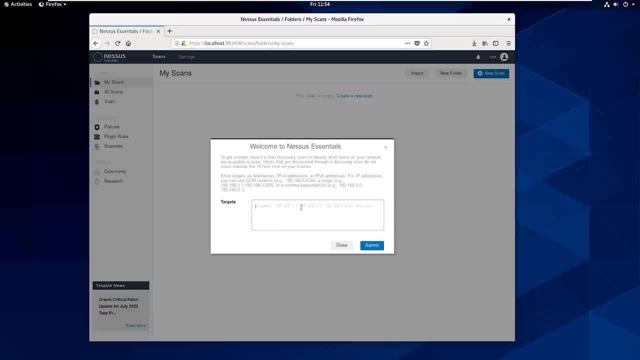 to discover all the hosts on our network. So I'm actually only going to scan the local host, because that's the system right now that I'm running this on. So I'll enter the IP address and hit submit And Nessus will go ahead and scan for potential hosts. It finds my host. So if we used a full 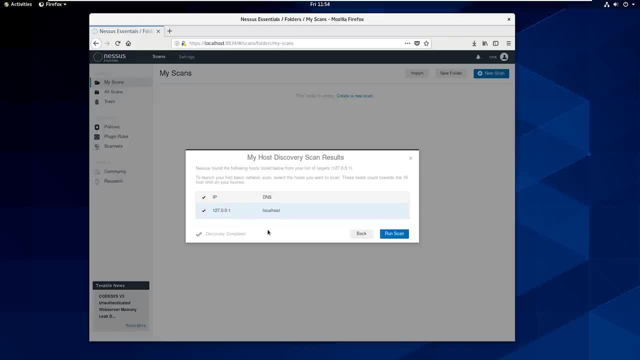 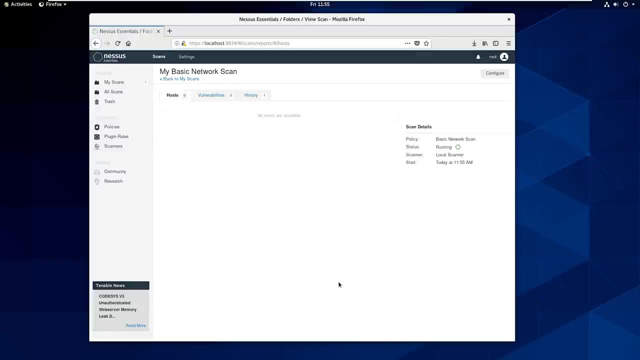 network or many hosts, and it would obviously list them in here. But again, with this home license you only have a 16 host limit that you can scan And then we will hit run scan, All right, and this is going to do a basic network scan. 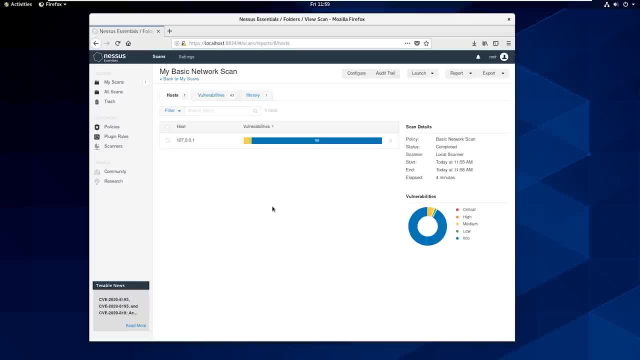 All right, now that scan is complete So we can actually drill down into the different vulnerabilities that it found. It will tell you some of the information early on, before it actually finishes, So you can look at the information before it finishes, But you can. 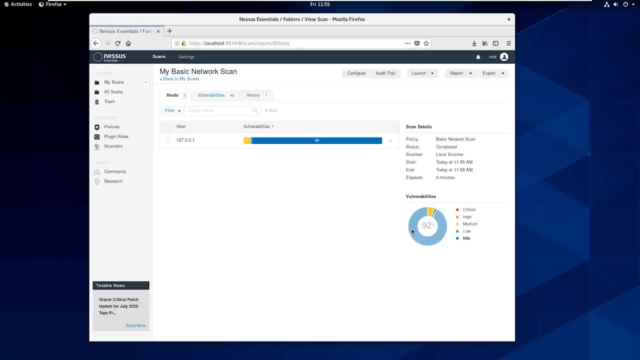 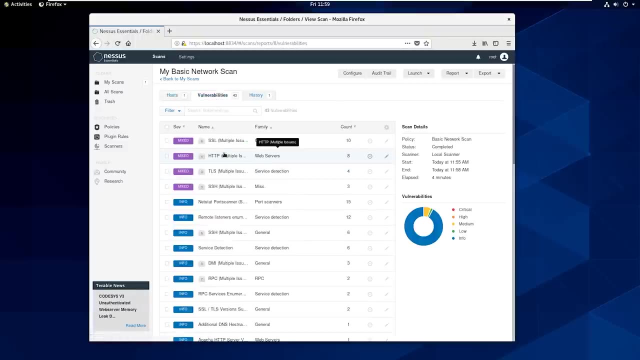 see here that we have this nice pie chart here. 92% of the findings were informational, 6% were medium, 2% were low. So if we want to drill down into that, we can go up here and click the vulnerabilities And it will tell us the individual issues. 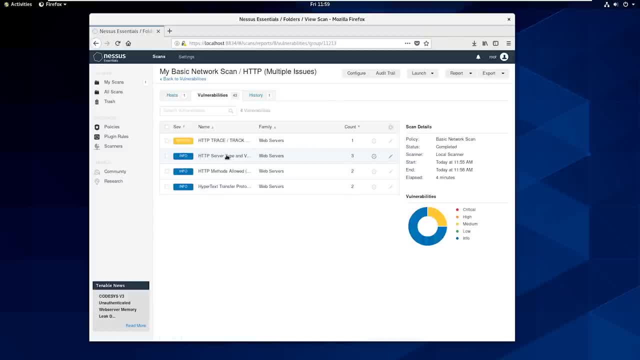 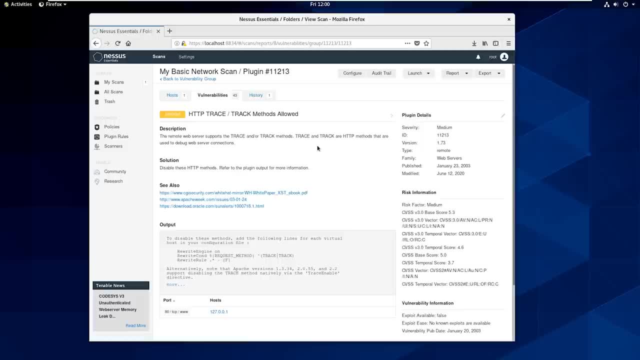 So we're going to go into this HTTP issue here And we can see there's a medium vulnerability And we're going to click on that one. You can see that it gives more information about that individual vulnerability and what it found. So in this particular one, this remote web server, 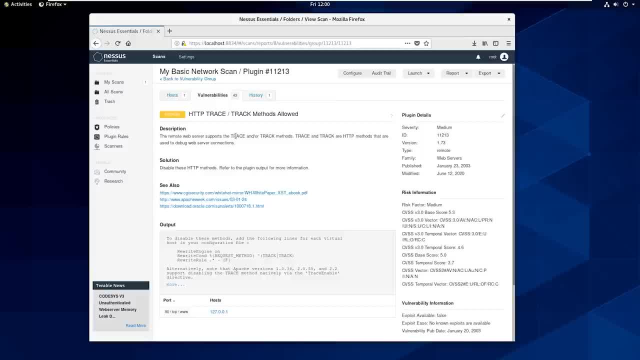 supports the trace and or track methods. With this I just installed a default instance And this is going to have some of these regular default findings in this vulnerability finding And you can also see this output, So it gives more information about it. 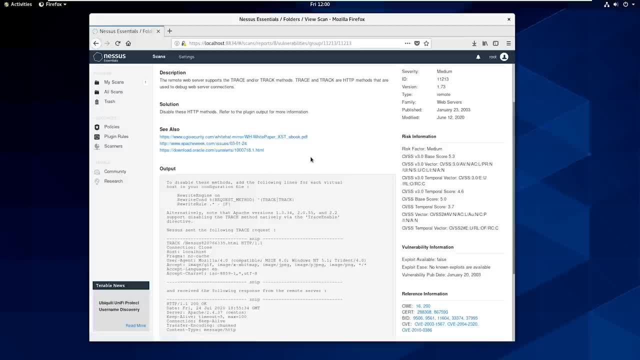 And you also get some article links that you can go check out as well. The medium rating, or the medium risk is based on what Nessus believes it is Okay, so that's where that medium comes from. And then you also get modified and the published date So you can see when they updated the signature. 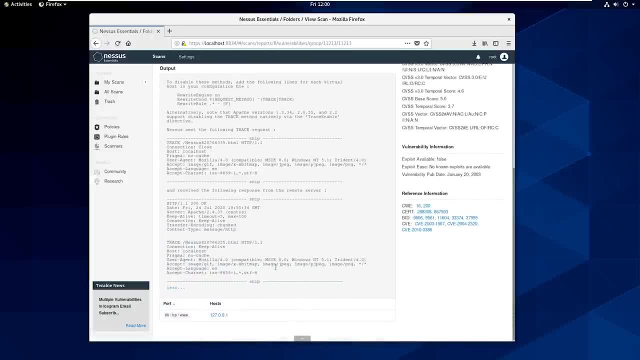 and just a little bit more information. You also get the port that it was found on, So ADTCP www- and the host that it was found on, So, again, local host, the system that I'm actually running it on Now. you also get some of these CVEs over here as well. 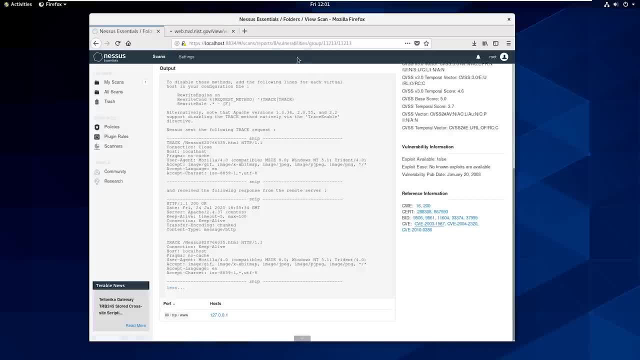 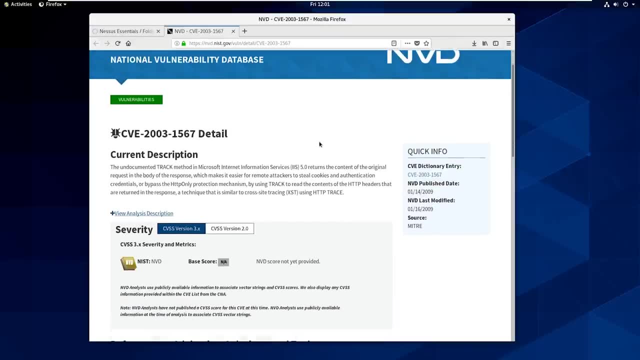 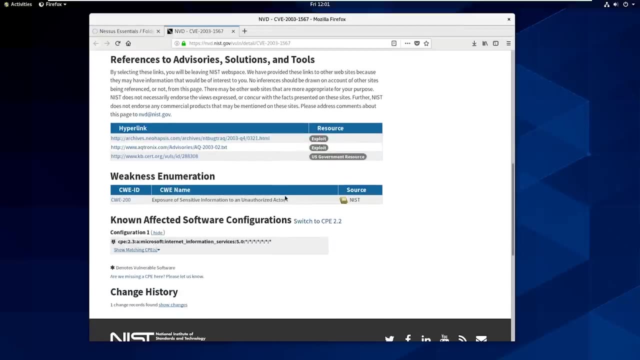 So if I click on this original one, go ahead and open that in a different window. that will take us to the actual database where it describes its findings, And I definitely would check this out. This is going to be a great database where you have a 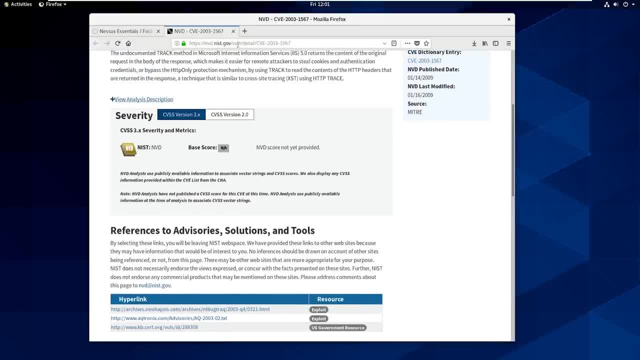 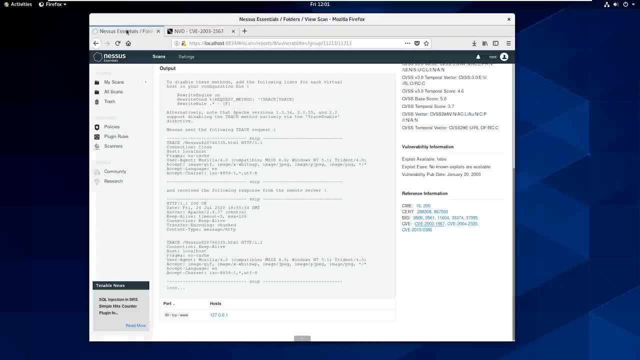 lot of different information. This is the NIST NVD website and this has all the different vulnerabilities that are out there. So and again, that was found on the original one For the specific vulnerability, the specific CVE. you found it on the actual vulnerability. 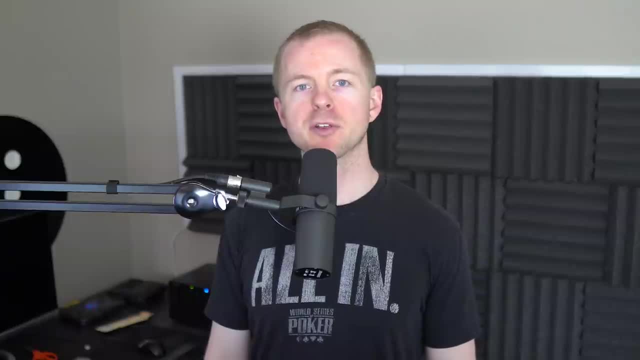 finding that links directly to it. When you're looking for more vulnerability information, you can also go to the vendor website because of course, they're going to release when there's a new patch and potential security issues, And that's in addition to what we can use on the scanner.